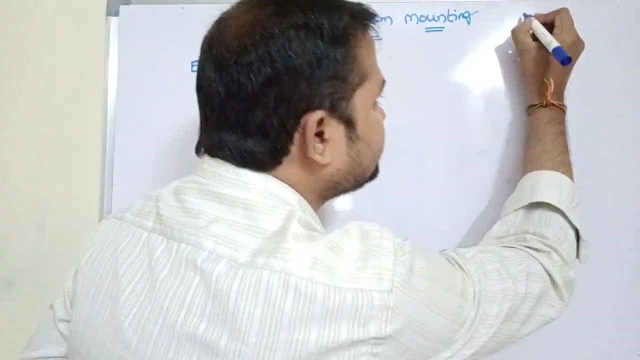 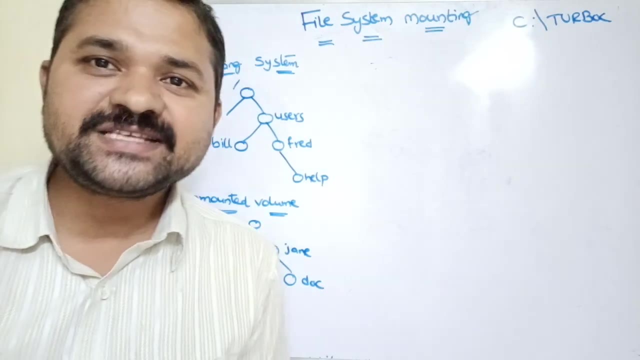 Let us assume that we have Turbo C In C. we have Turbo C, So by using Turbo C we can have Turbo C. So by using Turbo C we can have Turbo C, we can execute c file. but let us assume that we want to execute those programs from d. i want to. 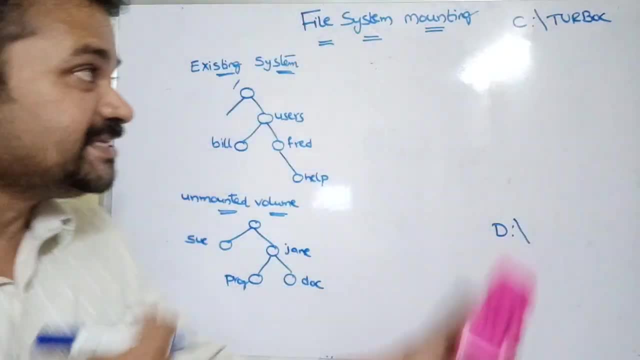 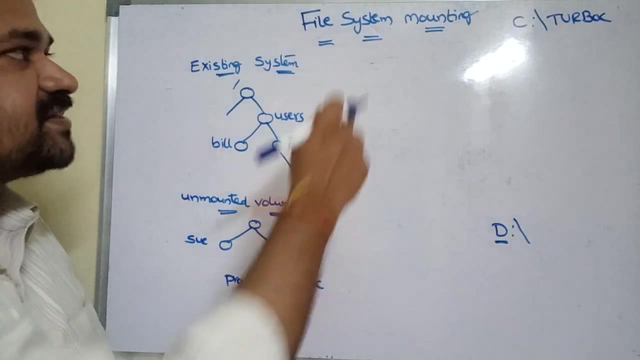 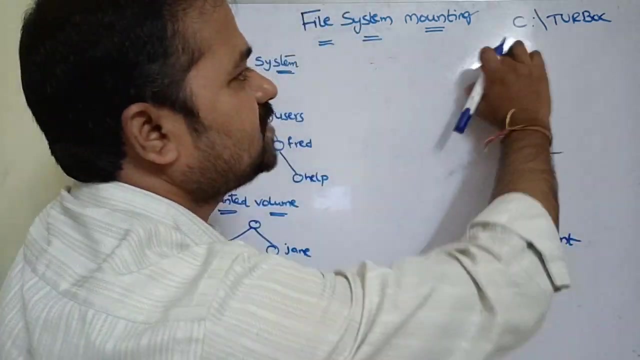 execute those programs from d, but turbo c is available in c, so we have to attach these files to the d file system. so for that we use a mounting. okay, so for that, simply, we use a command card mount space. so what is the files we need to attach here? c colon slash, turbo c. 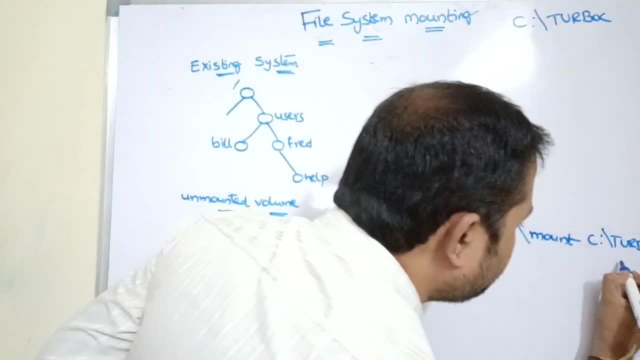 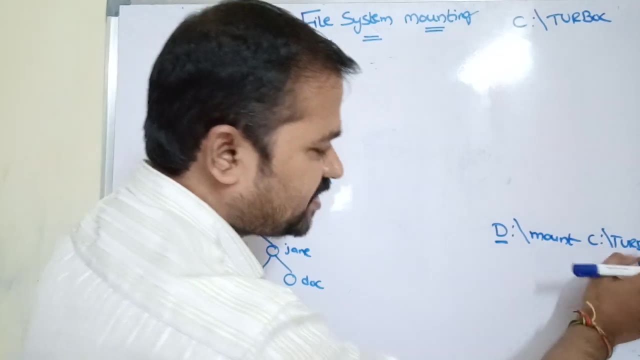 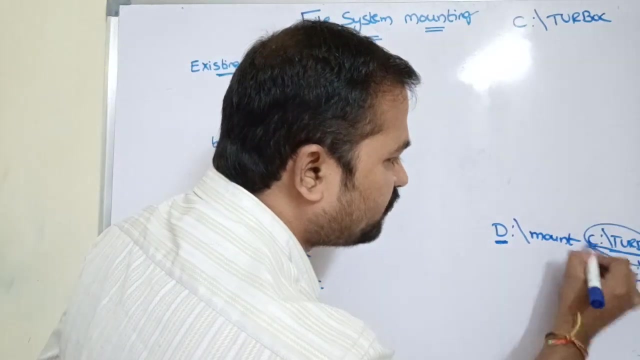 so at which part we need to attach it? d? so d colon slash. so whenever the statement is executed, then c colon slash, turbo c. so this turbo c folder will be available at d. so in d we can make use of turbo c directory files. so that is nothing but mounting. so mounting is a process, but 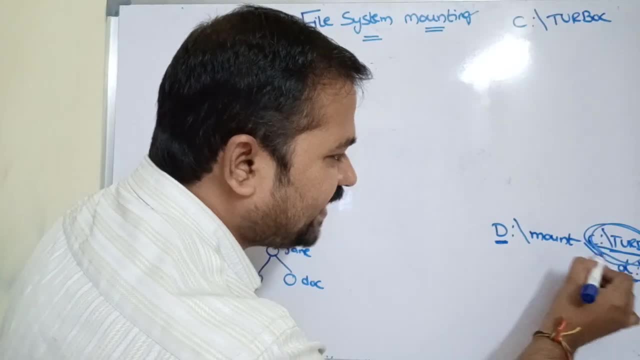 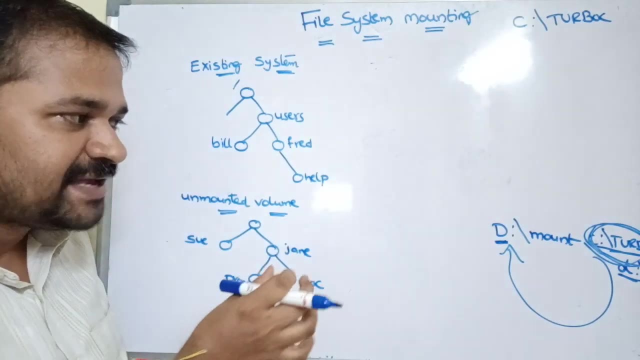 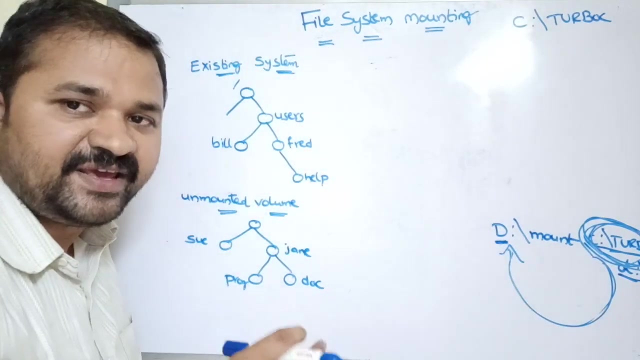 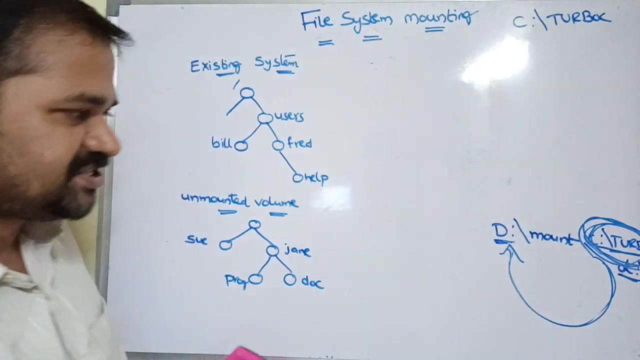 using which operating system makes files and directories available to a specific path. so here operating system is making available, making turbo c folder files available to d file system so that we can use this turbo c files yet d, so we can execute c programs from d file system. so this is about what is mounting a various unmounting means. 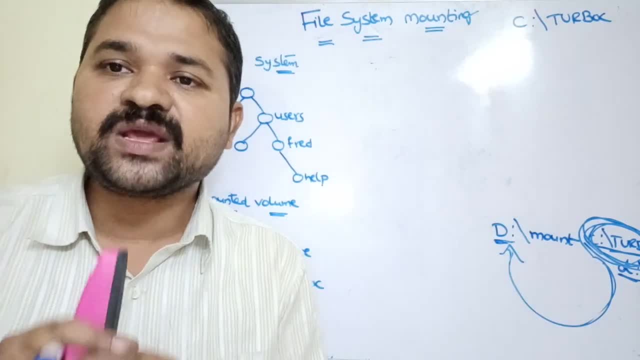 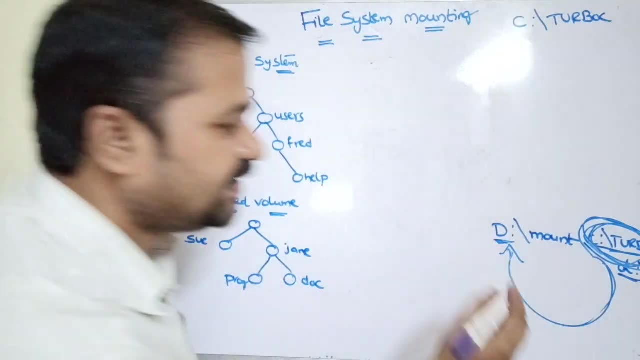 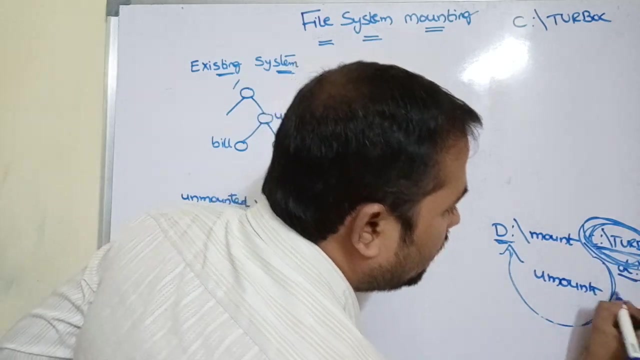 detach- detaching files from the file system. so removing files from the file system, so that at this path we don't have c colon slash turbo c files. in order to perform the unmounting we use a command called u mount, so u mount space. so what is the file system we are detaching? what is the folder? 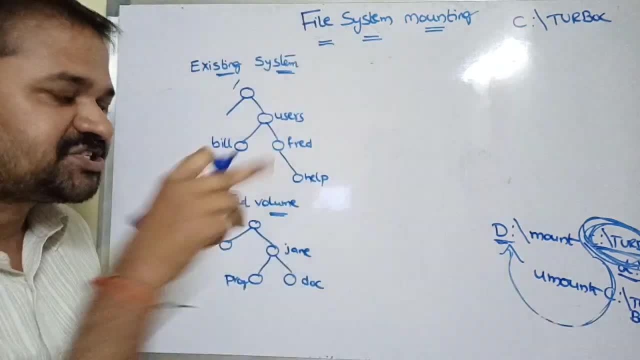 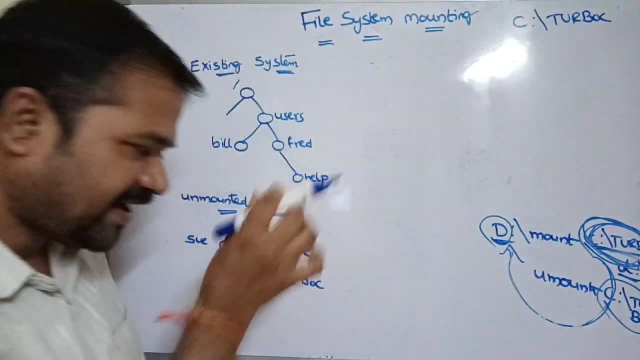 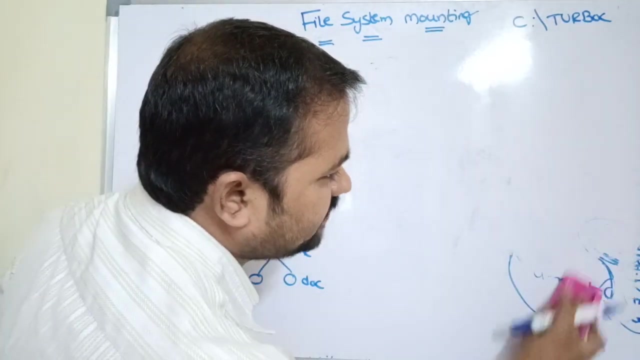 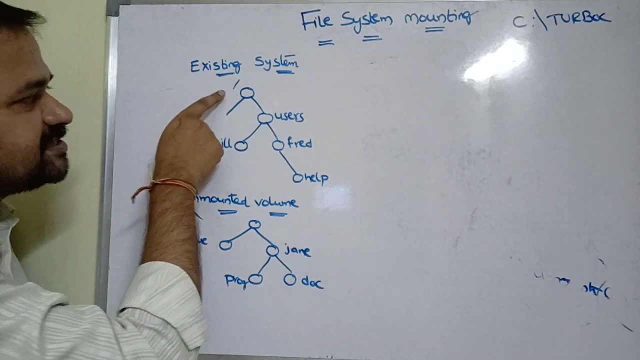 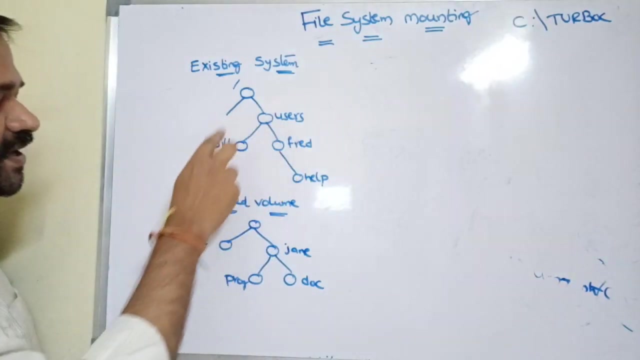 so u mount space c colon, slash turbo c so that this turbo c folder will be detached, will be removed from this d file system so that we can use this turbo c folder to do the unmounting so auto. so this directory contains a subdirectory called users. again, user subdirectory contains two.